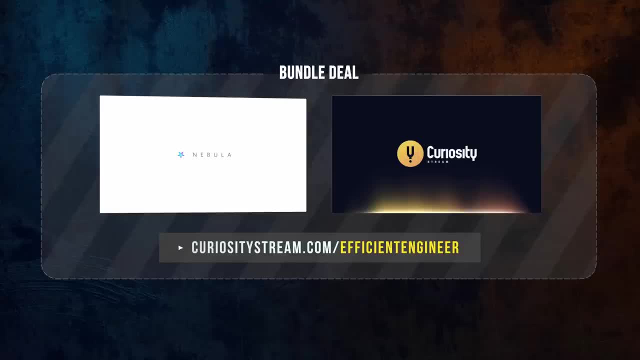 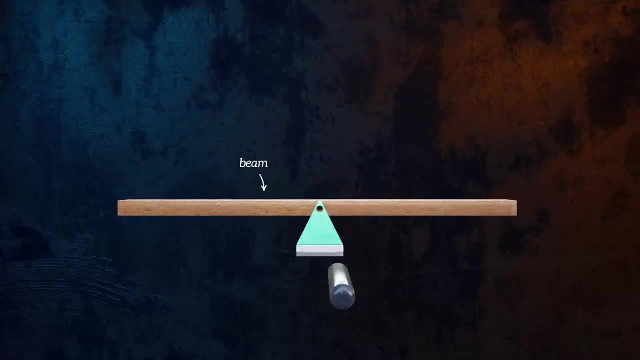 sponsor CuriosityStream, but more about that later. Let's start with the lever Consisting of just a beam pivoting about a fixed hinge called the fulcrum. it's one of the simplest ways of generating mechanical advantage. Consider the amount of force we need to balance a mass located at one end of the beam. 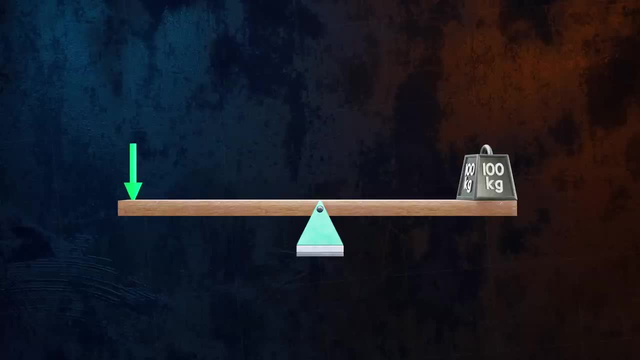 When discussing levers, it's common to talk about a load, which in this case is the mass, and an effort, which is the force that needs to be applied to lift the load. It's quite obvious that this system, with the fulcrum in the middle of the beam, 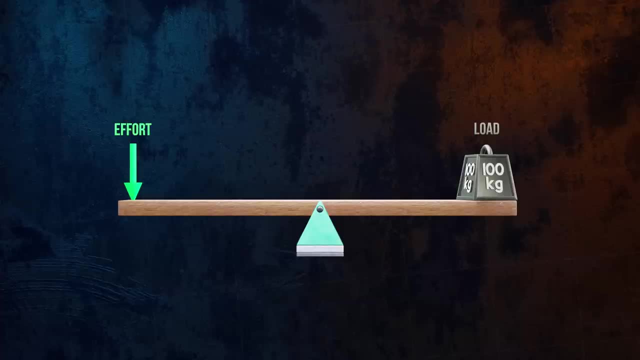 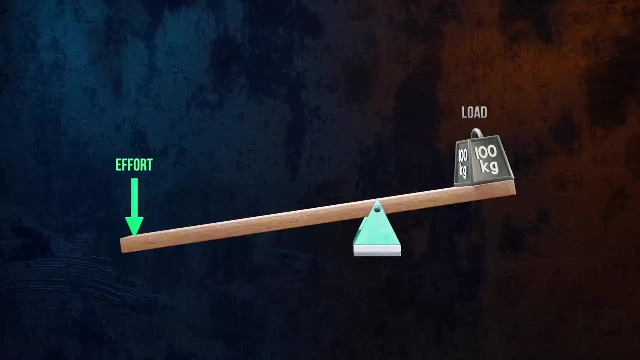 can only be balanced if the effort is equal to the load. But what if we move the fulcrum away from the center of the beam towards the mass? We now only need a much smaller effort to balance the lever. But why? We can explain this by considering the rotational stability of the lever. 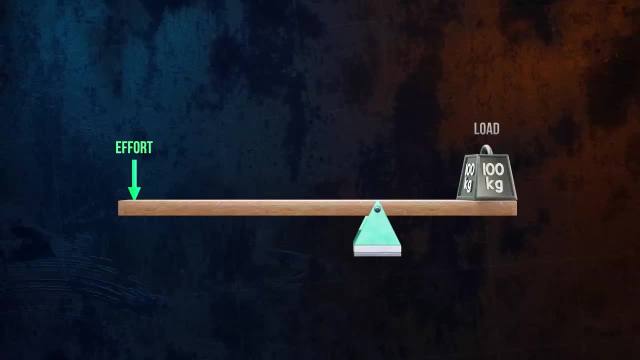 Both the load and the effort have the effect of rotating the lever, which means that they are generating moments about the fulcrum. A moment is a quantity that determines how much a force causes something to rotate about a specific point. It is calculated as the magnitude of the force multiplied by the 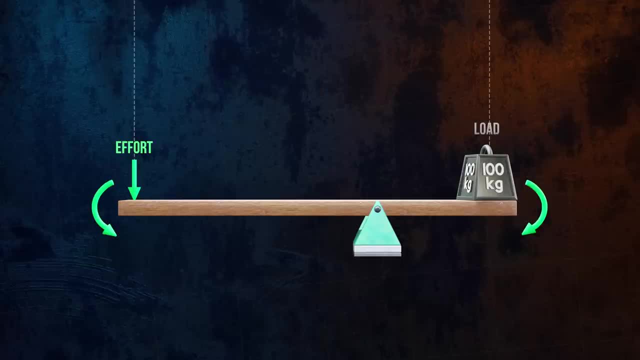 perpendicular distance from the line of action of the force to the point of interest. For the lever to be in rotation, it's necessary to have a force that is equal to the force of the lever In rotational equilibrium. the moments acting about the fulcrum must balance each other. 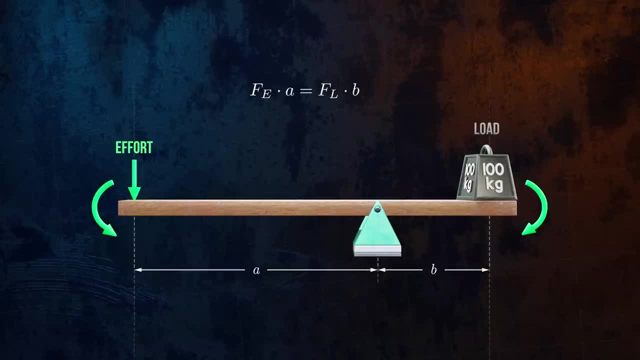 We can then easily calculate how large the effort needs to be to balance the load based on the distances A and B. Earlier we defined mechanical advantage as the ratio of the output to the input force. so we can see that for a lever it is calculated as the ratio of the two distances. 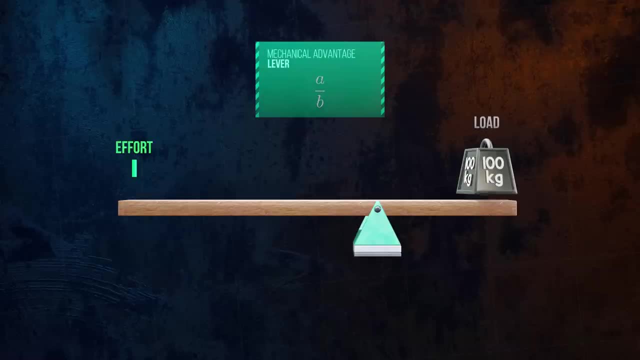 By moving the fulcrum we can change the mechanical advantage. Putting it very close to the load means we will be able to lift the mass with a much smaller force, which is incredibly useful. It might seem like the lever is somehow breaking the laws of physics. 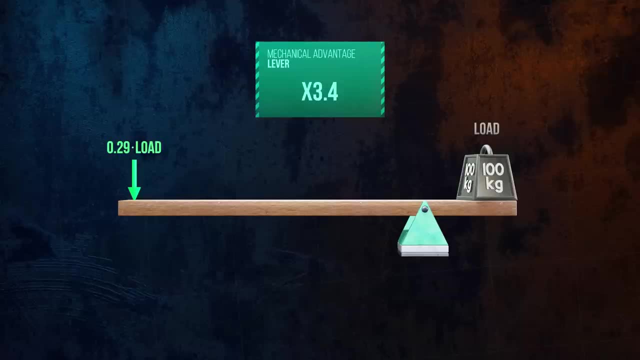 by turning a small force into a much larger one. but it's important to remember that levers don't actually create energy. The amount of energy used to lift a mass is equal to the magnitude of the applied force multiplied by the distance over which the force acts. 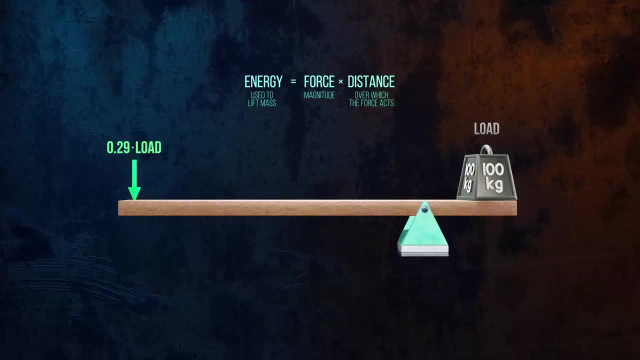 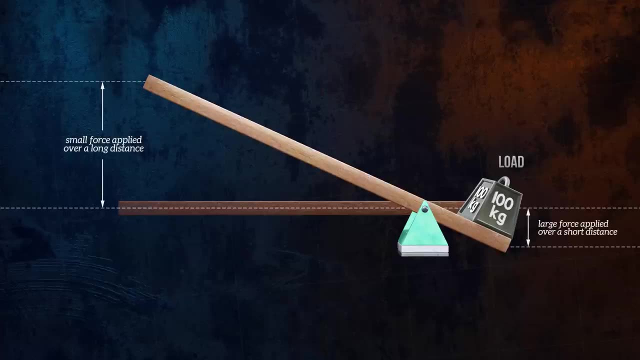 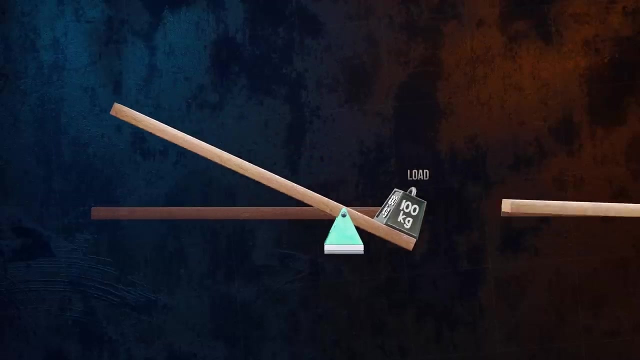 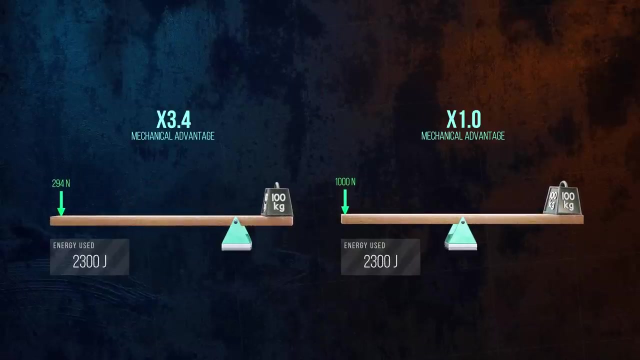 So although the force applied to lift the mass when using mechanical advantage is smaller, it needs to be applied over a longer distance. The amount of energy used is always the same, with or without mechanical advantage. All devices that generate mechanical advantage work on this same principle. 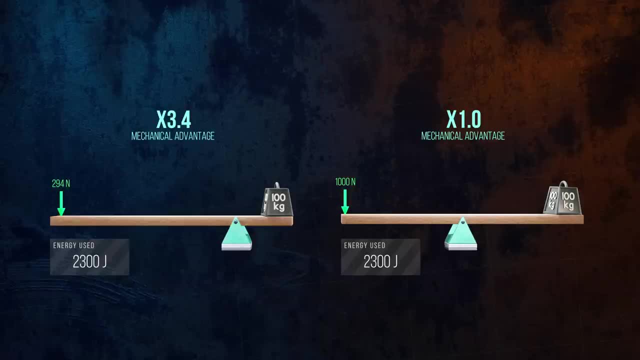 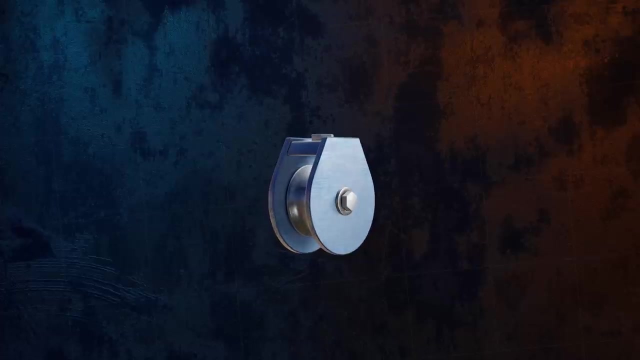 They convert a small force applied over a long distance into a large force applied over a short distance. The pulley, which is essentially just a wheel containing a groove through which a rope or cable can run, is a bit more difficult to understand than the lever. 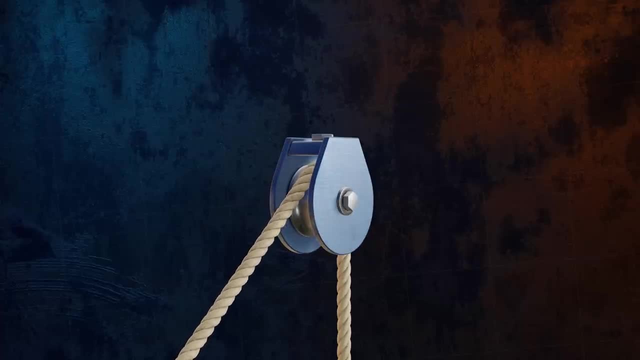 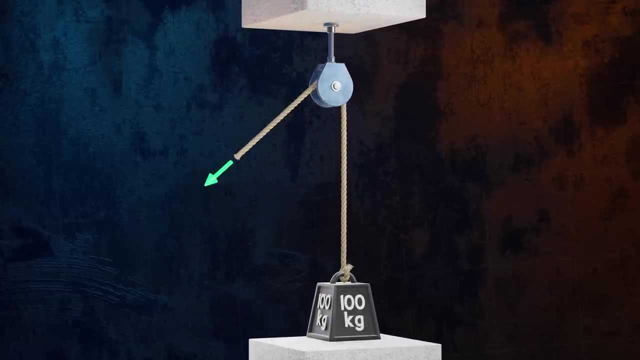 but opens up even more possibilities. Let's look at a simple configuration where a rope is passed through a single pulley and is attached to a mass. If a large enough force is applied to the end of the rope, the mass can be lifted. 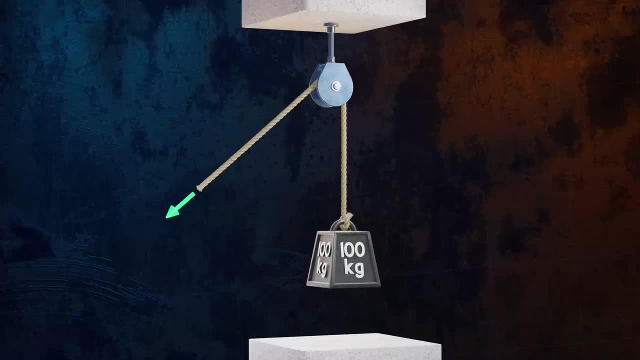 This system allows us to redirect the force needed to lift the mass so that we can pull on the rope at an angle instead of having to lift the mass vertically off the ground, But it doesn't actually provide any of the necessary forces needed. However, the rope can be lifted up from the rope and the mass can be lifted up from the rope. 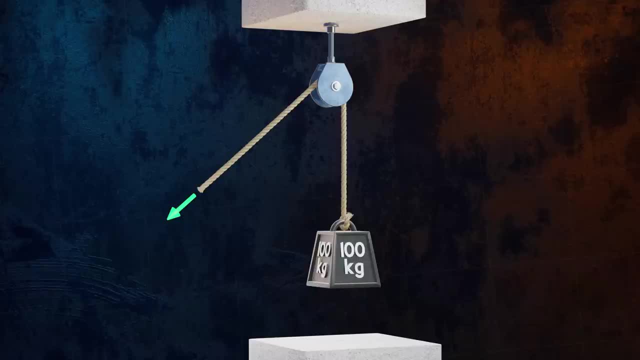 mechanical advantage. If the mass has a weight of one kilonewton, a one kilonewton force has to be applied to the end of the rope to lift it, Because the rope is being pulled on by the applied force at one end and by the 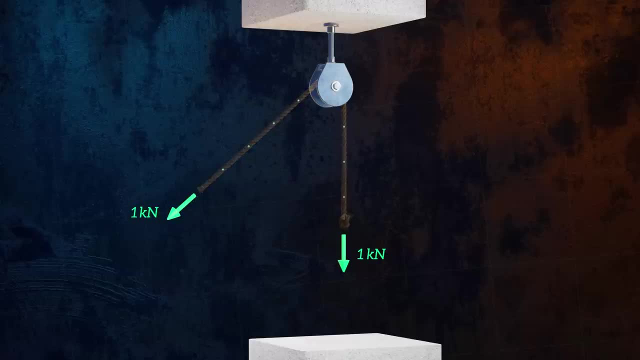 weight of the mass at the other, it's subjected to a tensile load of one kilonewton along its entire length. In reality, a slightly larger force will need to be applied to compensate for friction at the pulley, But to keep 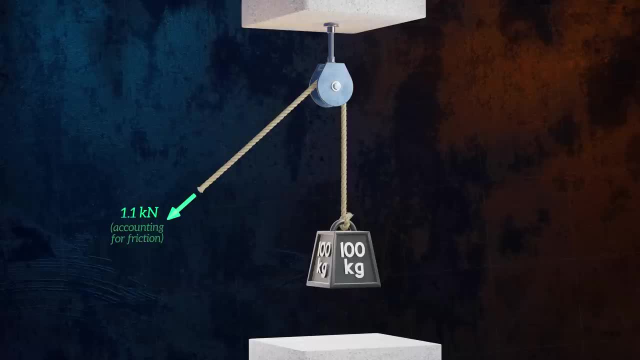 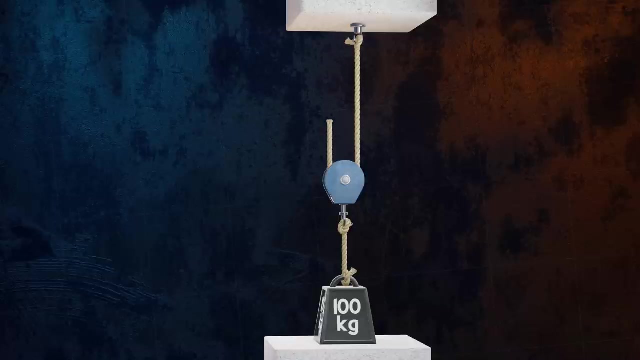 things simple. we'll assume that the pulley is both frictionless and massless. Let's look at a different setup now, where the pulley is flipped upside down and is attached to the mass instead of the ceiling. This small modification completely changes how the system works. It might seem impossible, but we now only 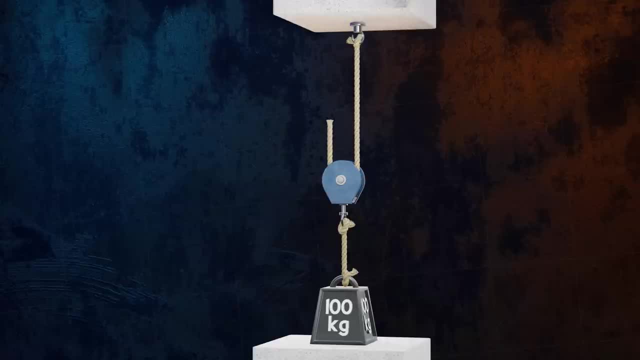 need to apply half the force we previously did to lift the mass. This system has a mechanical advantage of two. The reason is that the mass is now supported by two segments of rope instead of just one. To better understand what's happening, let's take a look at the forces acting on the pulley. 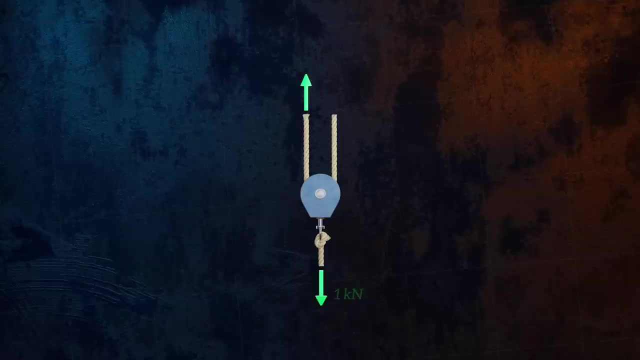 There is one downwards force, the weight of one kilonewton, and two upwards forces caused by the two parts of the same rope that are supporting the pulley. The tension in the rope is constant along its length, so the two upwards forces must 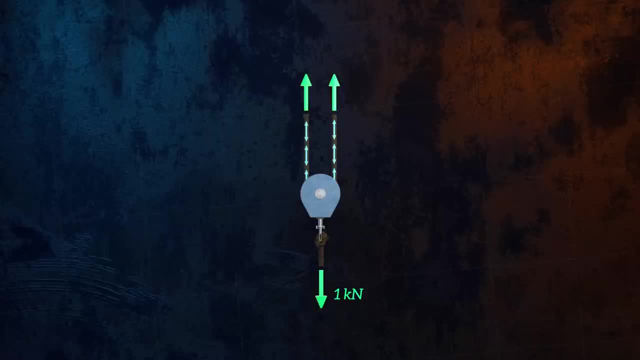 be equal to each other And for the system to be in equilibrium they must balance the one kilonewton load. We can conclude that both upwards forces are equal to point five kilonewtons. Since half of the load is taken by the ceiling, the load can be lifted by. 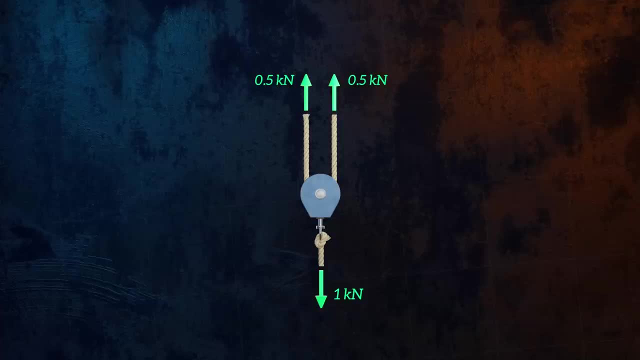 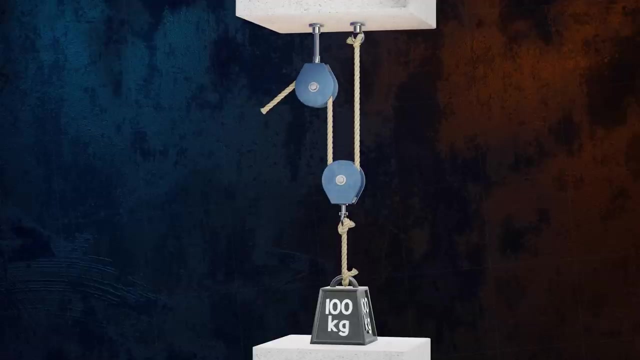 applying a force of only point five kilonewtons to the end of the rope. To make this system slightly easier to use, we can add a second pulley so that, instead of pulling up on the free end of the rope, we can pull on it at an angle. 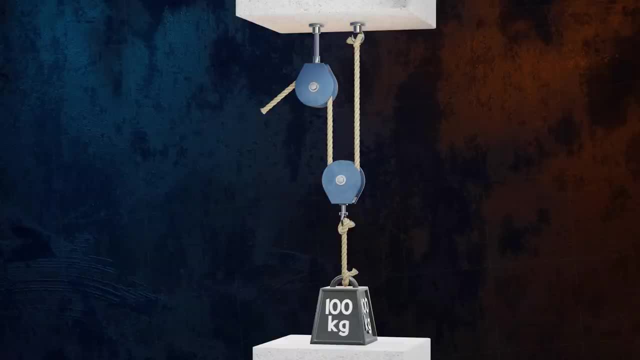 Like with the lever, the cost of dividing the force needed to lift the mass by two is that we have to apply that force over double the distance. The additional distance comes from the fact that two segments of the rope are already equal to point five kilonewtons. The additional license comes from the fact that two segments 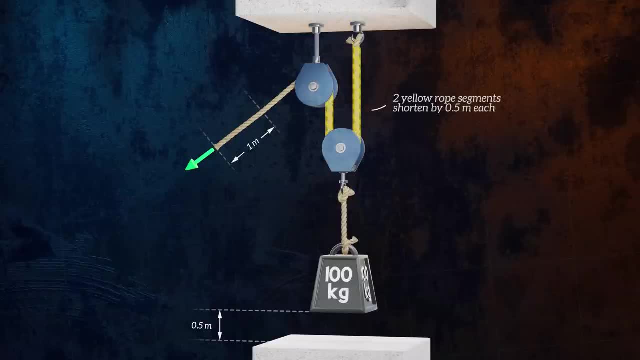 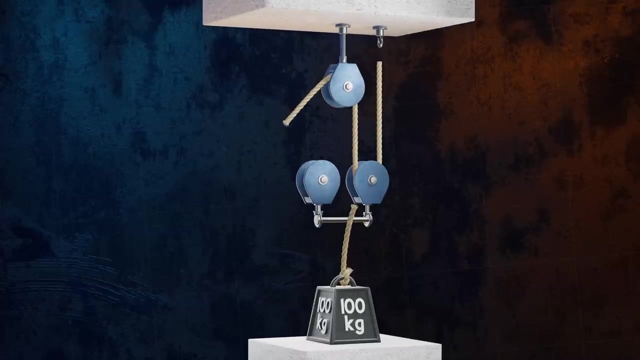 of the rope and nine kilonewtons are 2 kilowatts of a foot apart. contemporaneously, this makes rope need to be shortened to raise the mass instead of just one. Adding even more pulleys allows us to achieve greater mechanical advantage. 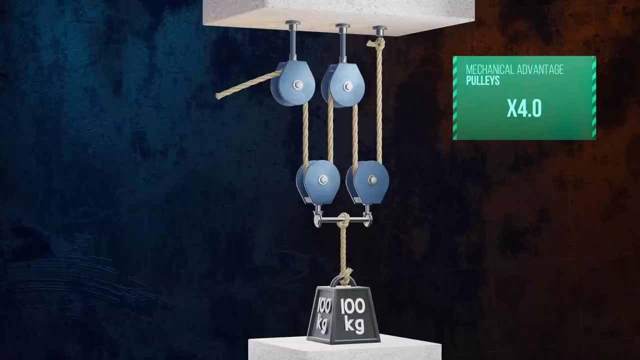 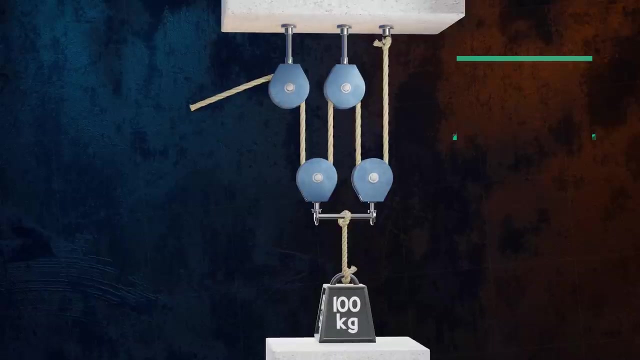 This system has a mechanical advantage of 4,. for example, The mass is supported by 4 rope segments. so producing an output force of 1kN only requires an input force of 0.25kN. Because using this many pulleys takes up a lot of space, the individual pulleys are usually 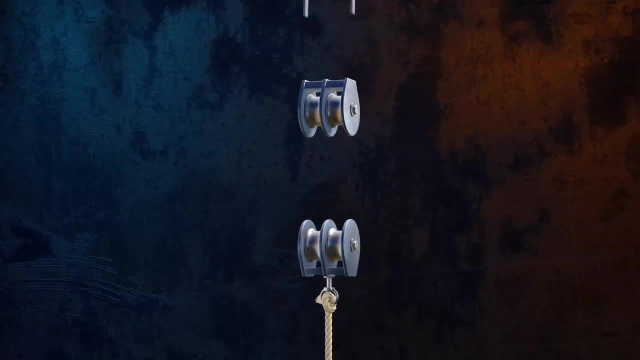 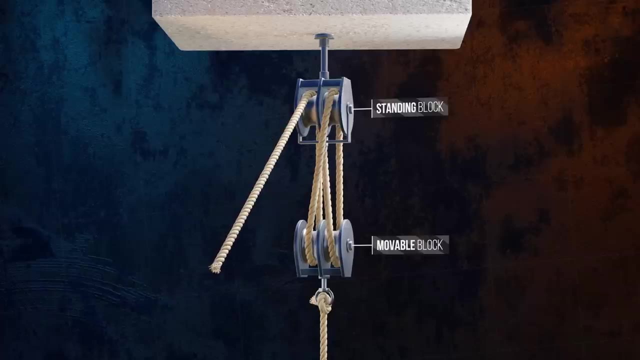 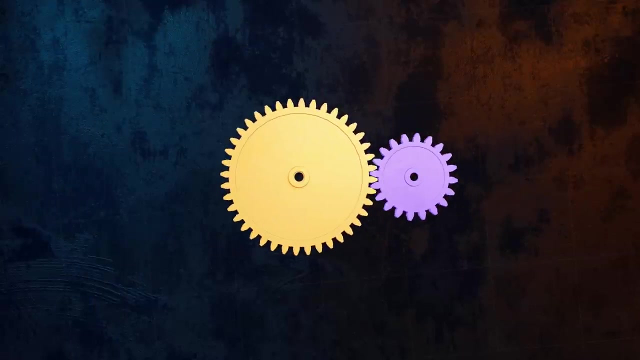 combined into two blocks: One movable block that moves with the mass and one standing block that is fixed to the ceiling. Gears are another type of simple machine that generates mechanical advantage. The teeth of one gear interlock with identical teeth on another to form gear trains that. 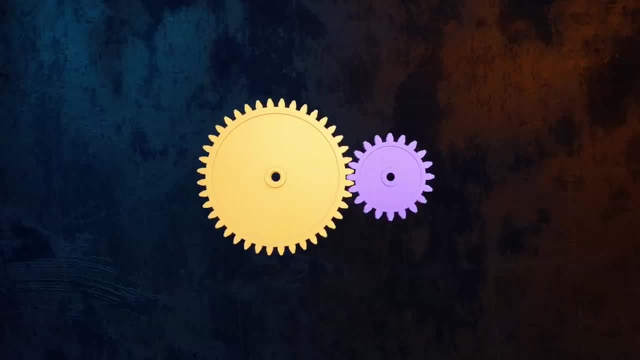 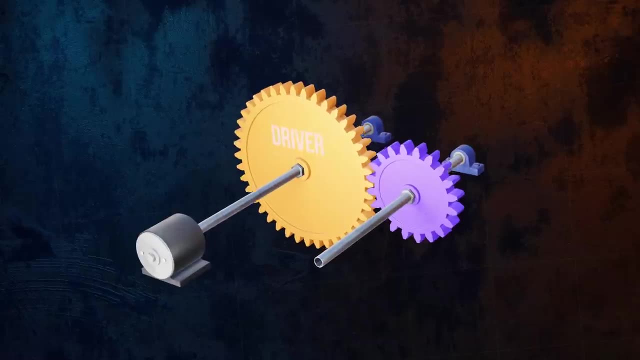 can be used to transmit and multiply forces. In each set of gears we can identify a driver gear that's connected to a motor or a rotating shaft and transmits force to a follower gear, causing it to rotate in the opposite direction. In this case, the follower gear, which has 20 teeth, is smaller than the driver gear. 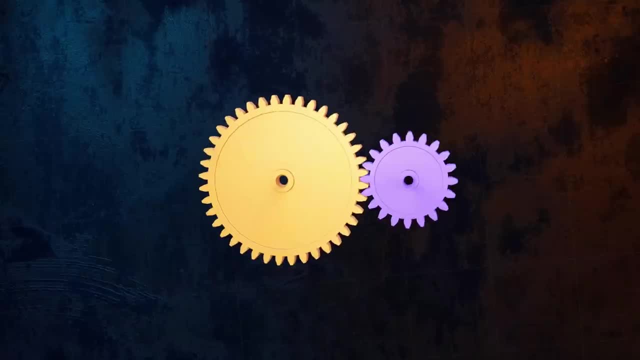 which has 40 teeth, For example in the part called�تي. in this example, Since the circumference of the larger gear is twice that of the smaller gear and the smaller gear must rotate twice for every one rotation of the large gear, 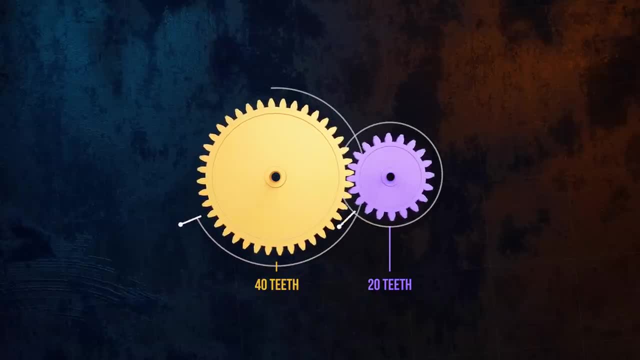 This configuration is called a speed multiplier. The follower gear is rotating twice as fast gear. To understand how gears can generate mechanical advantage, let's look at how force is transmitted through the system. This motor provides a torque of 100 Newton meters to the driver gear. 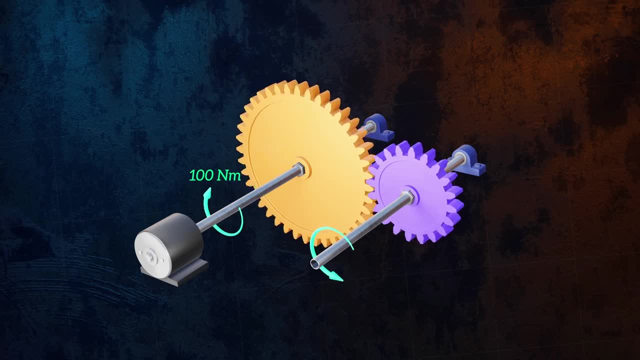 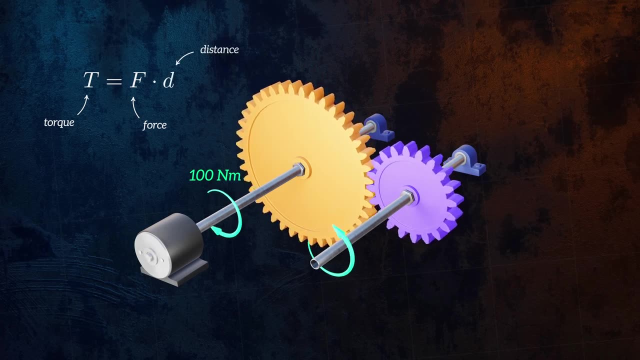 Torque is a moment that acts about a longitudinal axis and is calculated as the magnitude of the force multiplied by the distance to the axis of rotation. The torque of 100 Newton meters is equivalent to someone turning the shaft with a force of 100 Newtons at a distance of one meter, or a force of 200. 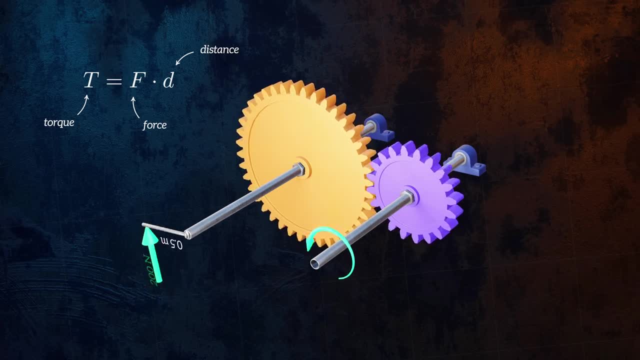 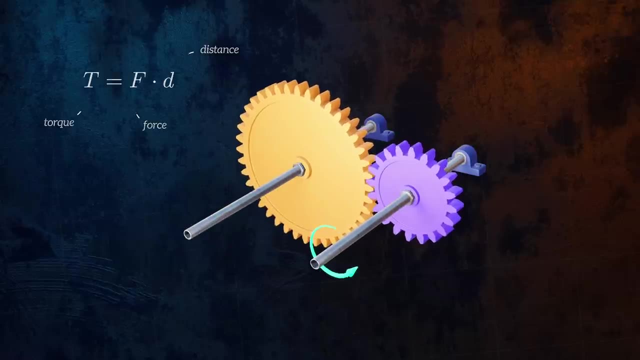 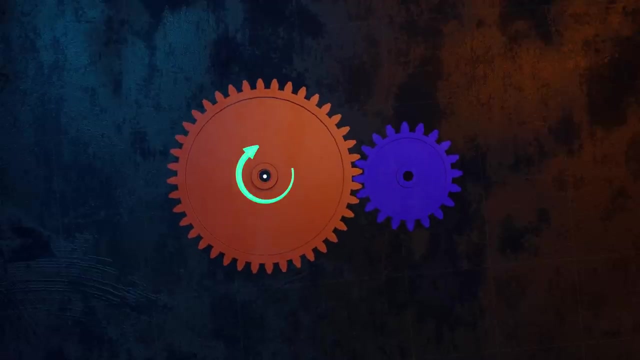 Newtons. at a distance of half a meter, for example, The input torque causes the driver gear to rotate, generating a tangential contact force between the two gears. We can calculate the magnitude of the contact force as the input torque divided by the distance between the force and the axis of rotation, which is 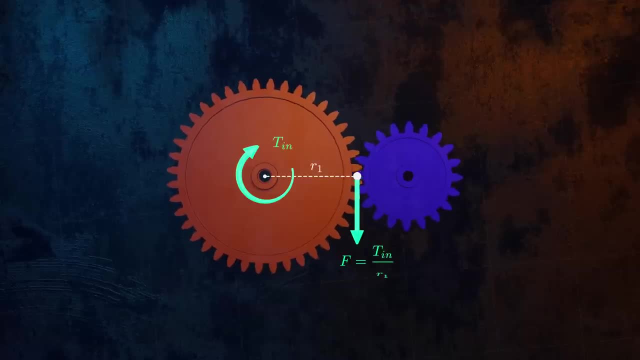 just the radius of the driver gear. The contact force causes the follower gear to rotate, generating an output- torque- that can be calculated as the product of the contact force and the radius of the follower gear. This tells us that the contact force can be calculated by the distance between the force and the axis of rotation. 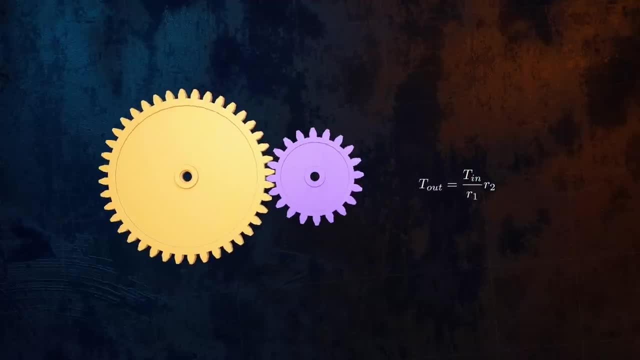 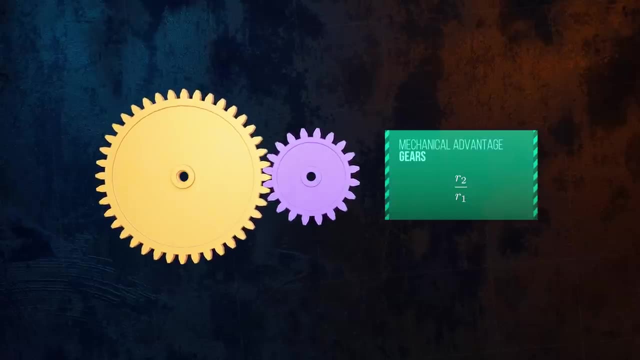 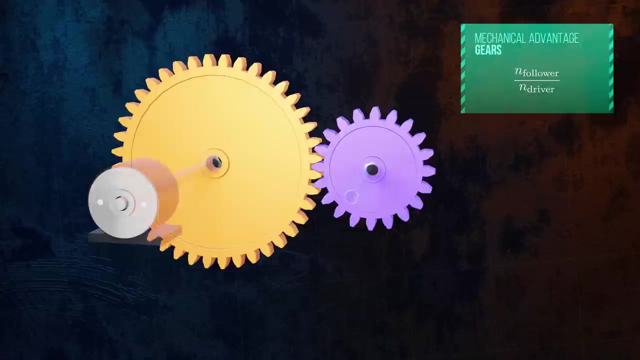 The mechanical advantage of this system is given by the ratio of the radii of the two gears. This is the same as the number of teeth on the follower gear divided by the number of teeth on the driver gear, With 40 teeth on the driver gear and 20 on the follower gear. this particular 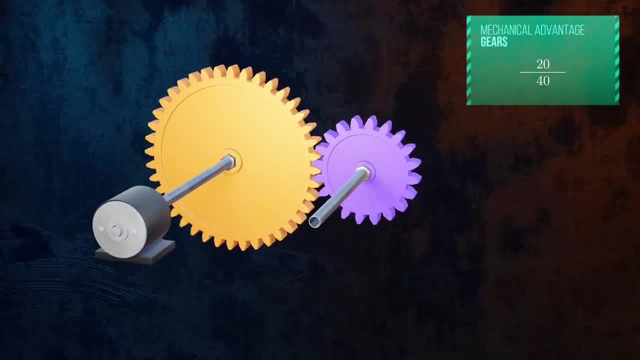 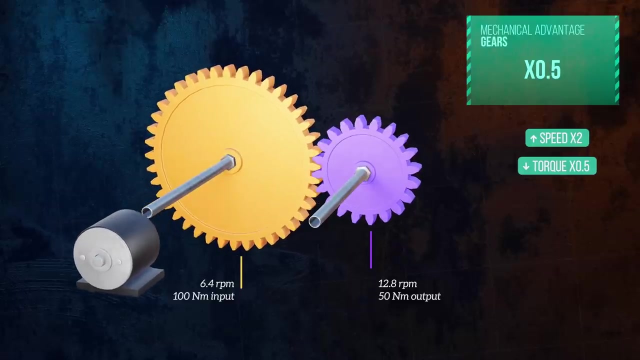 system has a mechanical advantage of 0.5.. Doubling the speed of the follower gear comes at the cost of halving the output torque. but if the smaller gear is the driver gear, the system will have a mechanical advantage of 2. The output. 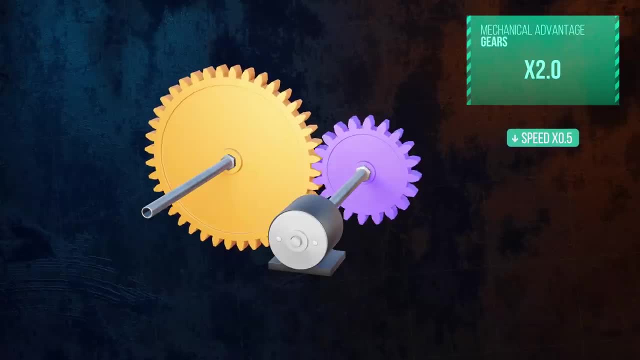 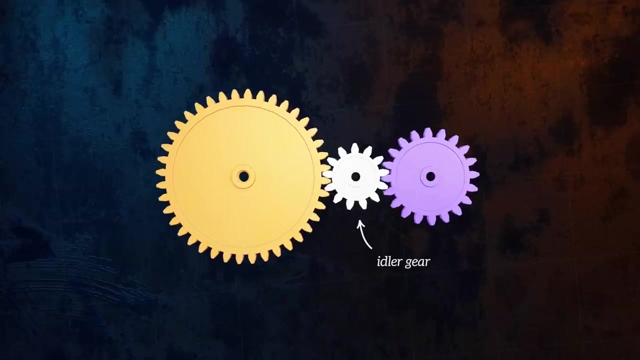 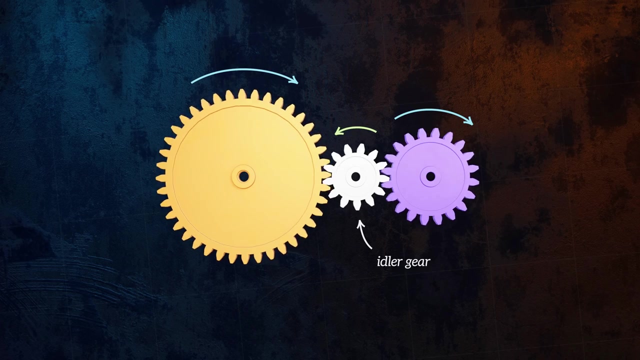 speed is halved, but the output torque is double the input torque. Even when a system has more than two gears, the mechanical advantage only depends on the number of teeth on the follower gear. This means that a third gear can be added to make the driver and follower gears turn in the same direction without affecting the magical advantage of the system. 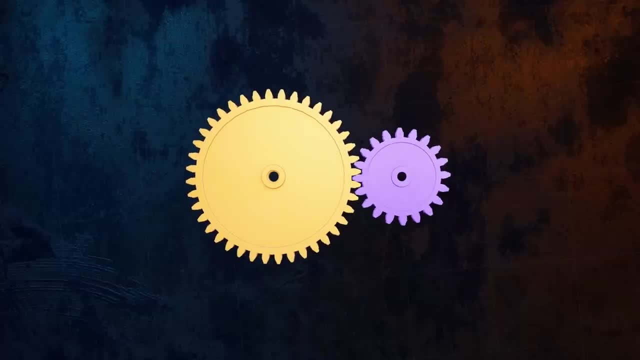 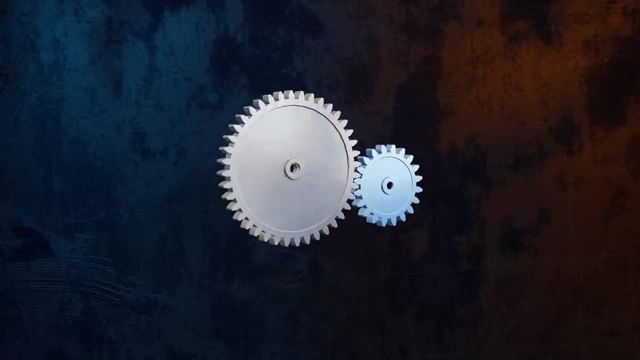 Using a small driver gear to turn a large follower gear and generate large ks is how a hand winch works. The Vega-B Kearns running gear contains a number of teeth with small Estudables within A drum around which a cable is wound is attached to the large follower gear. 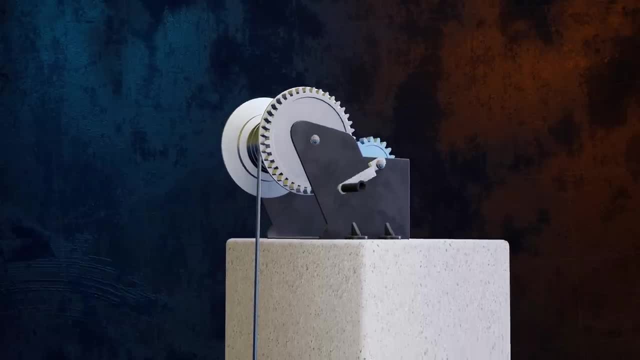 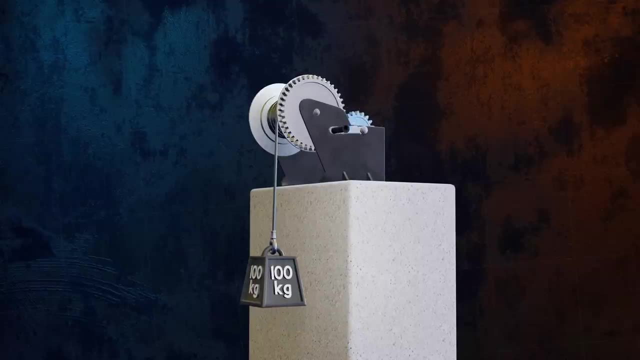 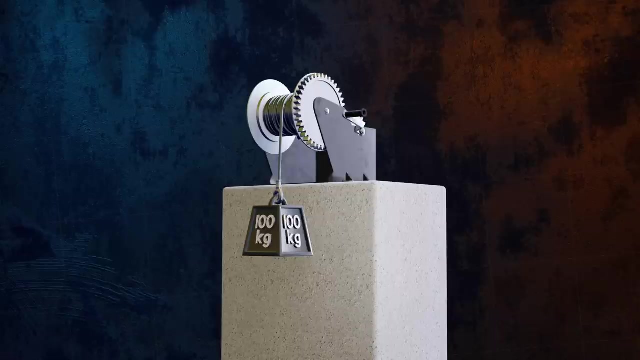 and the small gear is driven by turning a handle. The larger number of teeth on the follower gear means that the input torque from the handle is amplified, allowing heavy objects to be moved by the winch Levers. pulleys and gears aren't the only devices that can amplify forces. 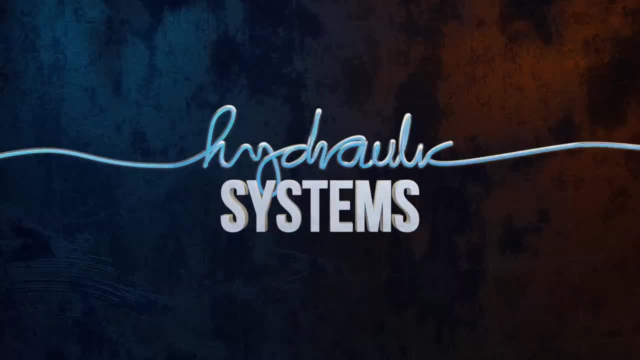 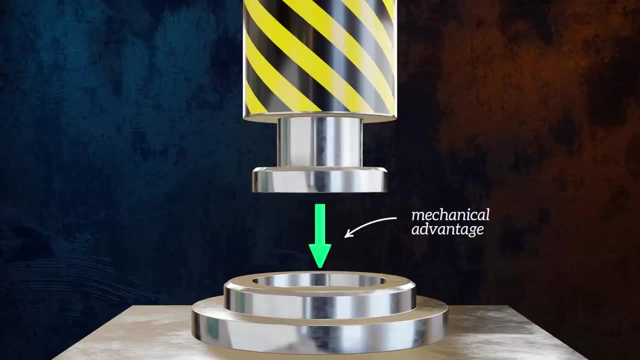 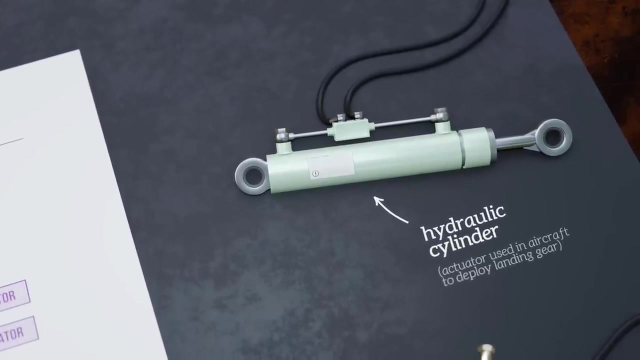 Hydraulic systems, like you would find in a hydraulic press, for example, use the incompressibility of liquids to generate mechanical advantage, which makes them useful for applications like the deployment of landing gear in aircraft flight control systems. If you're interested in learning more, I've just published a video on Nebula that goes into the. 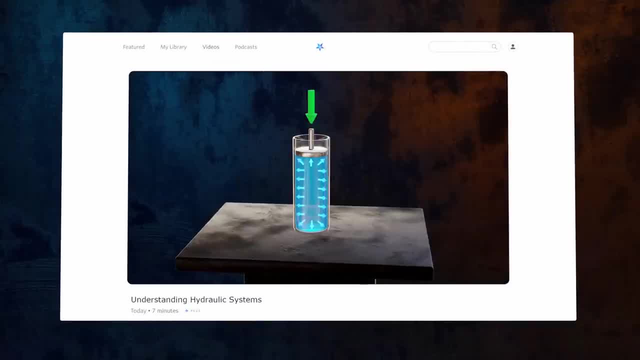 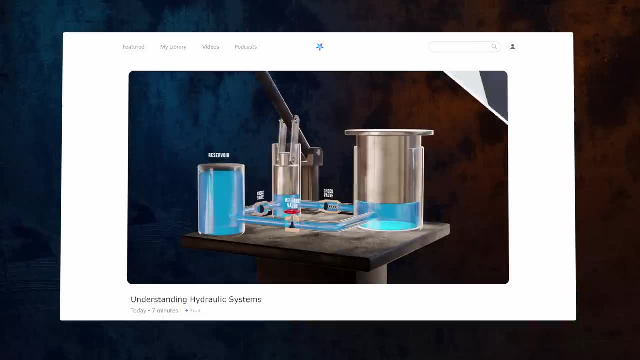 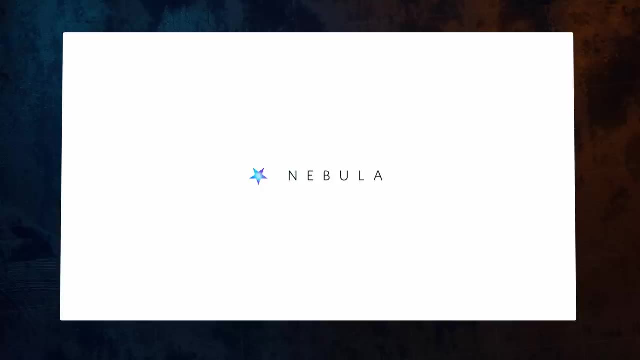 detail of how exactly hydraulic systems are able to generate mechanical advantage and the different components you need to build a functioning one. Nebula is a crater-built streaming site that's home to a growing collection of exclusive or extended efficient engineer videos, but also loads of ad-free content. 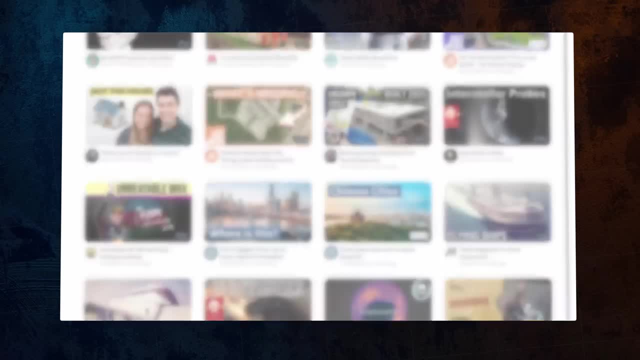 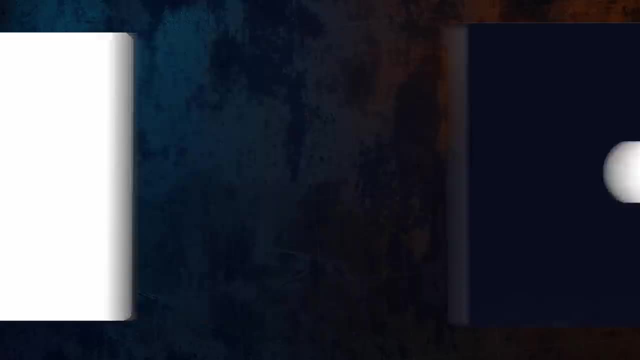 from over 100 of them. And here's the best part: you can get Nebula for free if you sign up to CuriosityStream, who have kindly sponsored this video, Where Nebula is the home of independent, thoughtful content. CuriosityStream is all about. 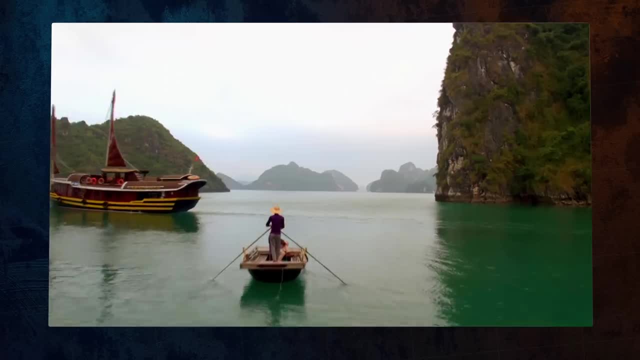 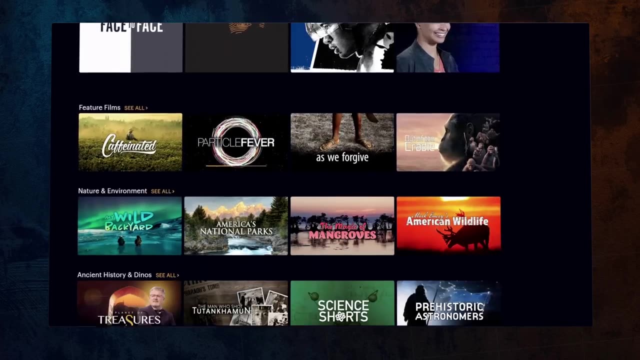 big-budget, high-quality documentaries and, with thousands to choose from, you'll always be able to find something interesting to watch. One excellent series I'm watching at the moment is Bridging the Expanse. It's a series that I've been watching for a long time. 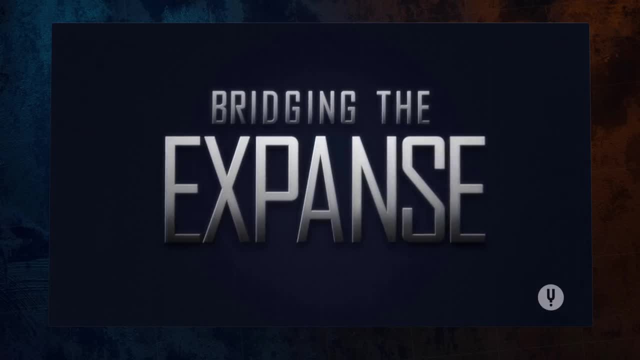 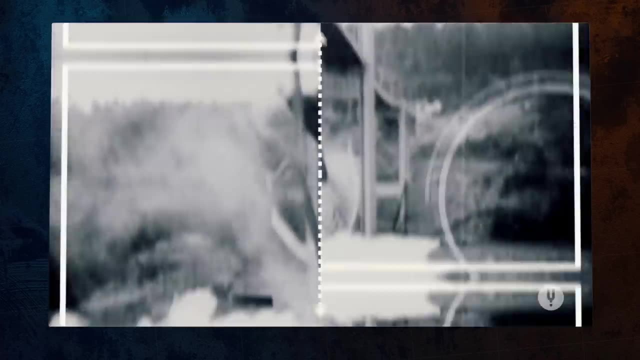 It's a great series With impressive animations and interviews with leading engineers. its six episodes celebrate the beauty of bridges, highlighting the most spectacular and innovative bridge designs and charting how the form and function of bridges have changed as bridge materials have evolved. 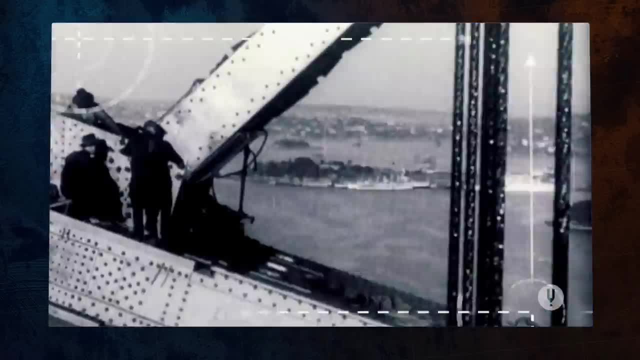 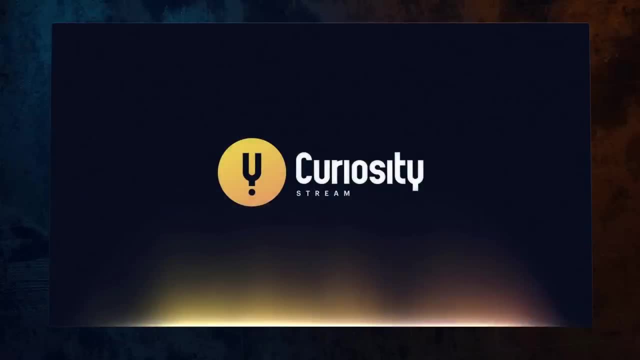 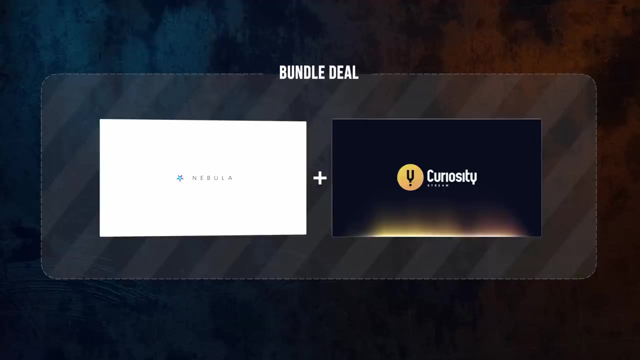 from wood to stone, stone to iron and iron to steel. It's just one of many great documentaries on CuriosityStream. With the CuriosityStream and Nebula bundle deal, you get access to a wide variety of content and you get access to thousands of amazing documentaries on CuriosityStream.